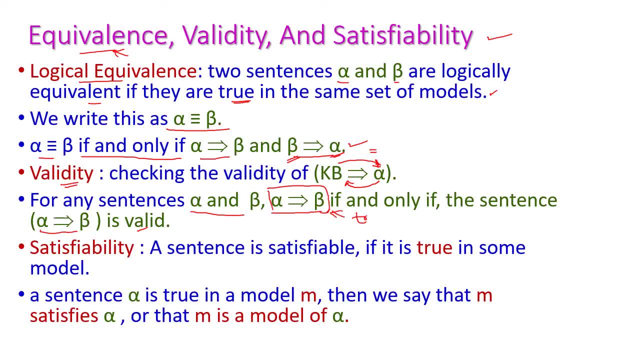 is alpha implies beta is true, alpha implies beta is true, then we can say that this particular statement is valid. right, and next one is satisfiability. here the validity and satisfiability are very much similar. that is, the sentence is satisfiable if it is true in some model. 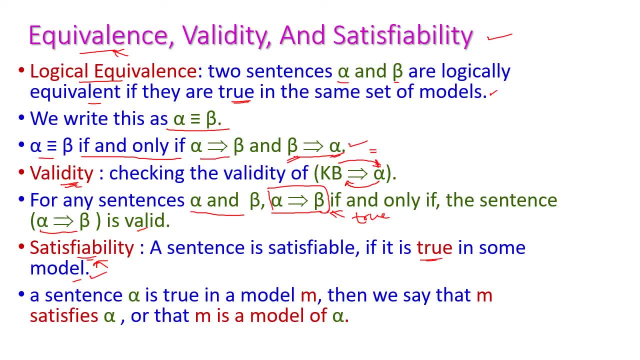 if it is true in some model- for example a sentence alpha- is true in model m, then we can say that m satisfies a, m satisfies a or m is a model of a, m is a model of a. okay, when we said m is a model of you. 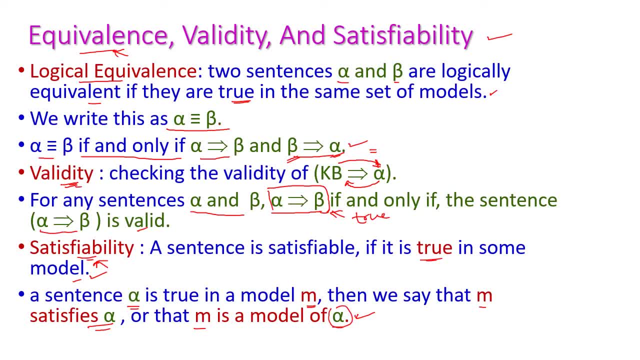 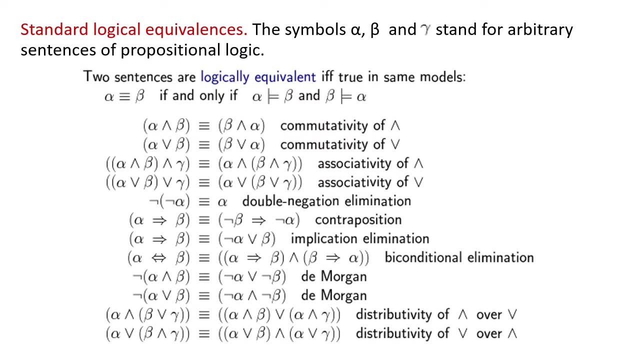 alpha. this is alpha, actually a sentence. If the sentence is true, then this particular sentence satisfies this particular model. And next let us see the standard logical equivalence. That is the logical equivalence here. Here we are using three different standards, that is alpha and. 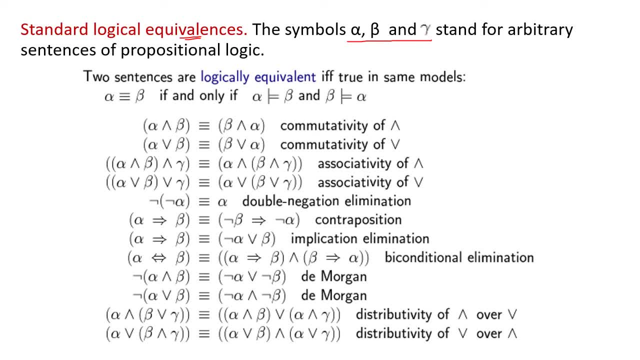 beta, gamma are symbols for a particular sentence of propositional logic. Here two sentences are logically equivalent: if, and only if, those sentence will be true in some model, For example, alpha is equal to beta, if, and only if, alpha entails beta and beta entails alpha, If both true, both these. 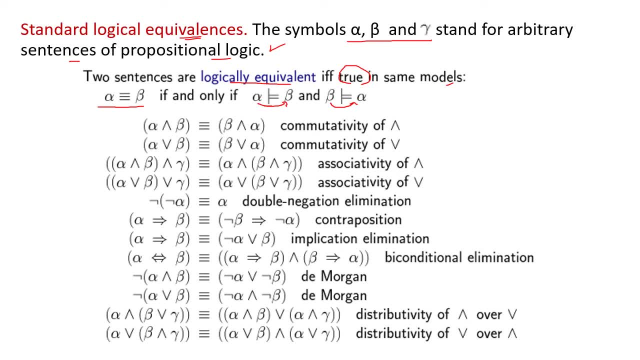 things will be true then alpha is equal to beta. Okay, so this is called as logical equivalent. Okay here. next come to commutativity law. that is, alpha and beta is equal to beta, and alpha, Alpha or beta is equal to beta or alpha. So this is commutative, and and commutative are 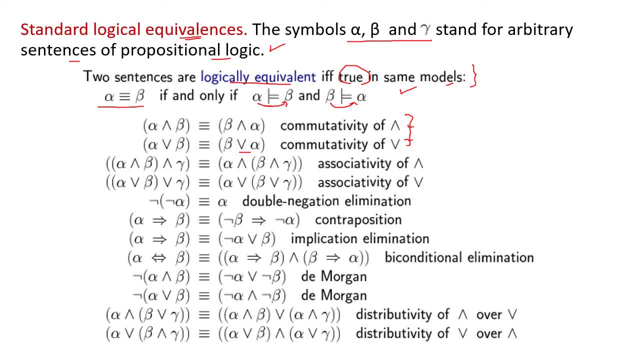 And next one is associativity law, Here associative and is alpha and beta and gamma are equal to beta and alpha, So this is commutative and and commutative are. And next one is double negation: elimination here, Now negation of negation: alpha. 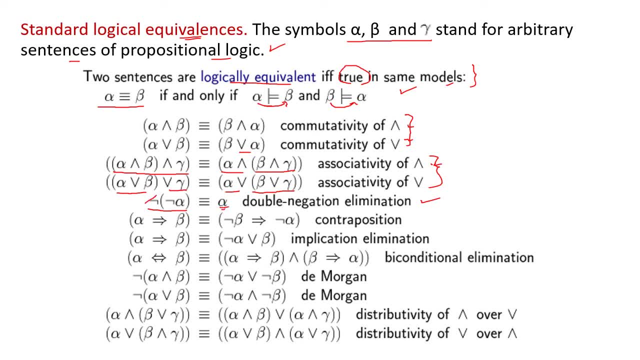 which is equal to alpha. that is, we need to remove these two negation. This is double negation elimination and the next one is contraposition. here alpha implies beta, which is equal to not. beta implies not alpha, not beta implies not alpha, right, so this is contraposition. 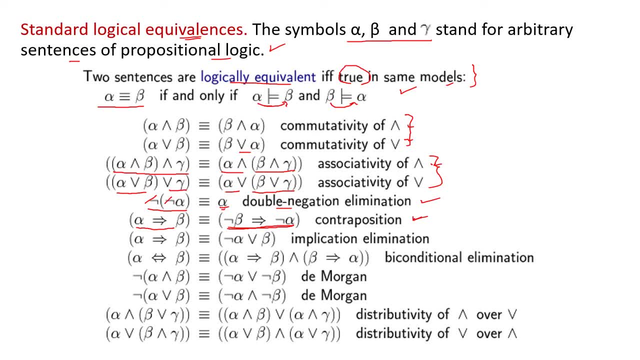 and next one is implication elimination. okay, that is, we need to eliminate this particular implies operator- alpha implies beta, which is equal to not alpha or beta, not alpha or beta. so this is implication elimination. and next one is biconditional elimination. biconditional elimination: we have to remove this particular operator, alpha, biconditional beta, which is equal. 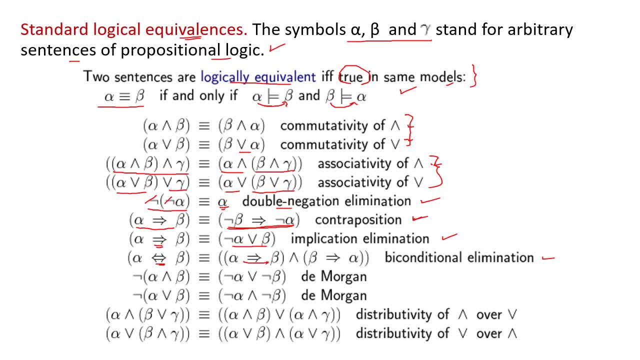 to alpha implies beta and beta implies alpha. so we remove this biconditional operator here. And next we come to the De Morgan's law. Here negation of alpha and beta is equal to negation of alpha or negation of beta. And next one is negation of alpha or beta is equal to negation of alpha and negation of beta. 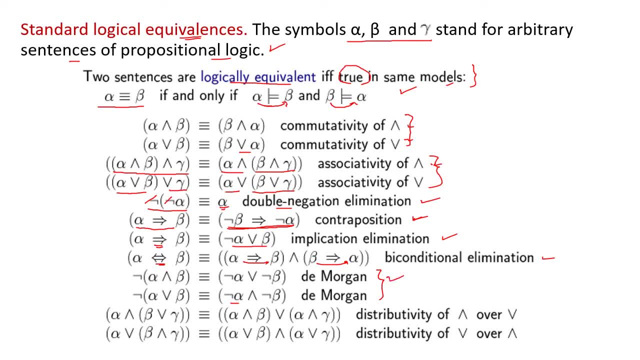 Okay, so this is De Morgan's law And next one is distributivity of and over r and r over and law. Okay, distribution law here. Here, alpha and beta are gamma, which is equal to alpha and beta are alpha and gamma. 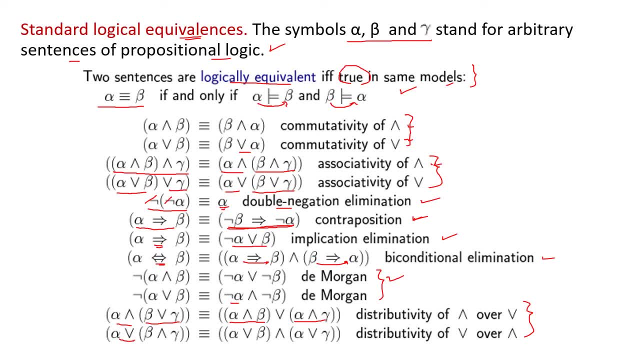 And next one is: alpha are beta and gamma, which is equal to: alpha are beta and alpha are gamma. So this is distributivity of and over r and r over and law. Okay, so these are the very famous standard laws. You might have studied all these things in your TOC subject, or distributivity, computer subject itself, Right? 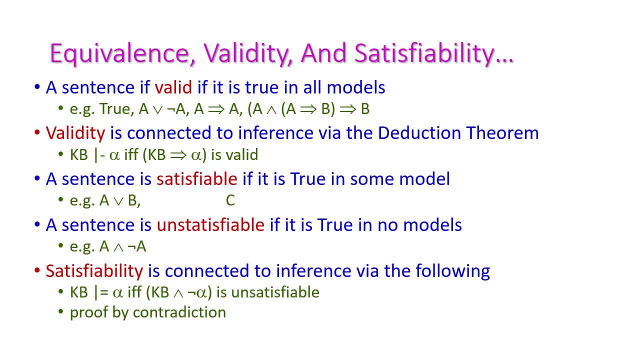 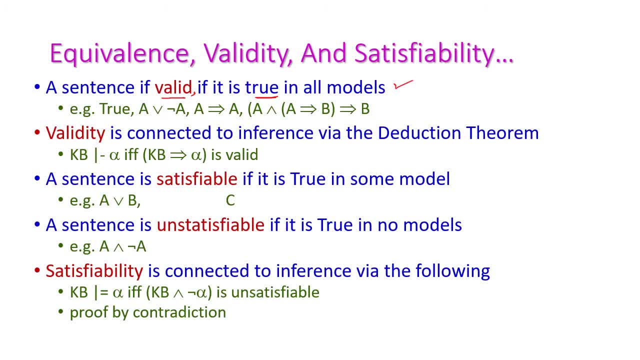 can accept that particular sentence is valid. for example, this one: a or not a, a or not a is always true. right: a implies a is also always true. and next one: a and a implies b, which implies b, this is also always true. okay, so these are all valid statements or valid sentences. 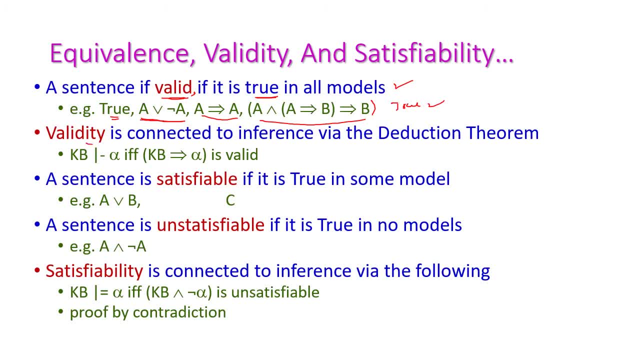 okay, here, validity is connected to inferences via deduction theorem. okay, here, knowledge base entails alpha. if, and only if, knowledge base implies, alpha is always valid. and when a sentence is satisfiable when we said, this is satisfiable if it is true in some model. okay, for example: 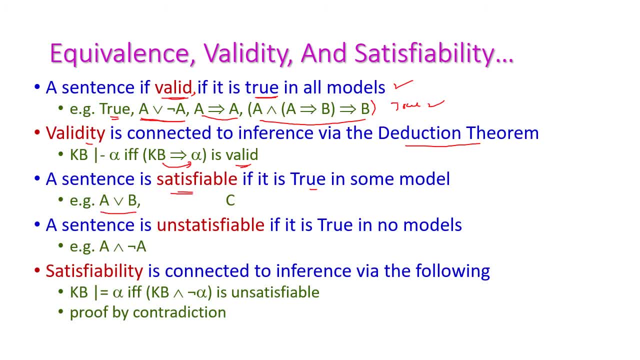 alpha and beta, which is equal to c here. if it is true, then this c is also true. right. and next one is: if a sentence is unsatisfiable, if it is true in no models, okay, so the situation Sentence will always give false value or negative value. 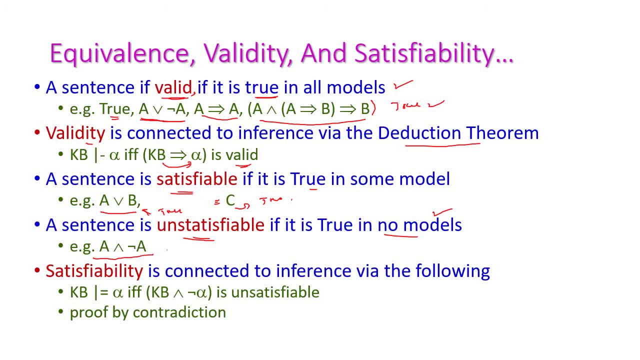 Okay, Here alpha and not alpha will give always false. So this is unsatisfiable statement. Satisfiability is connected to inferences via the following: That means the knowledge base entails alpha, if, and only if, knowledge base and not alpha is unsatisfiable. 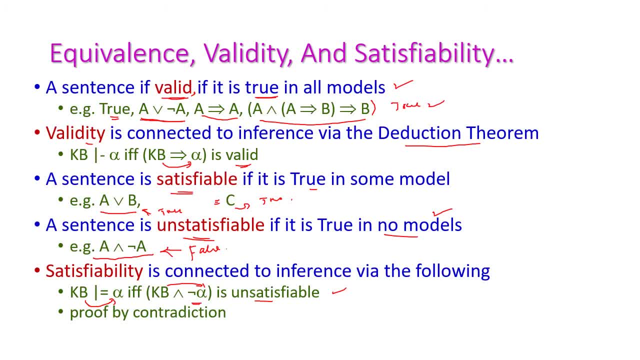 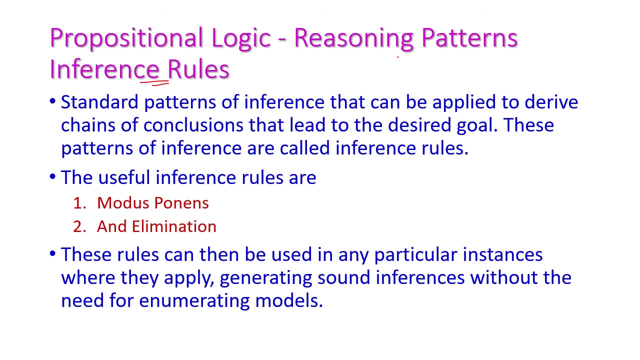 Okay. So if it is not alpha, then it will not be in this knowledge base. So this is proof by contradiction. That is the negative proof. Proof by contradiction, Okay, And the next one is the reasoning patterns. Here we are going to see the inference rules. 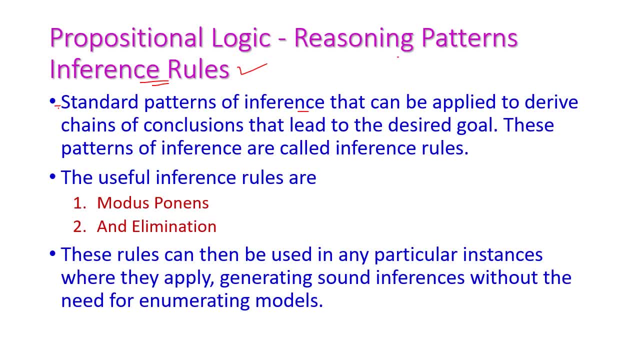 Here a standard pattern of inferences That can be applied to derive chains of conclusions, Chains of conclusions that lead to the desired goal, Right. And these pattern of inferences are called as inference rules. Right, That is, we are going to infer something from the standard statements which is in the knowledge base. 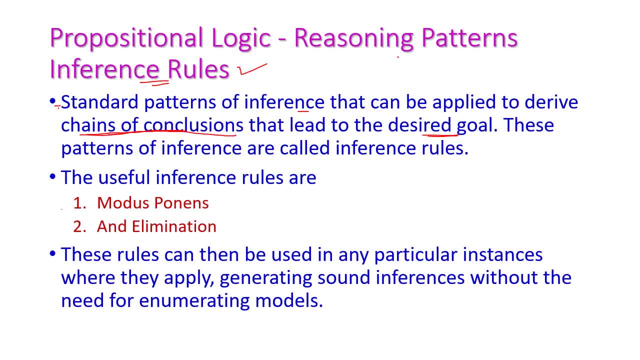 Right Here. the useful inference rules are: first one is modus ponens and second one is and elimination. This is and And and operator elimination Right. These rules can be used in any particular instance where they apply, generating sound inferences without the need of enumerating models. 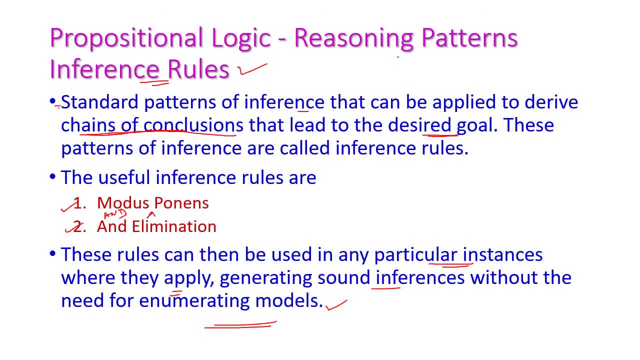 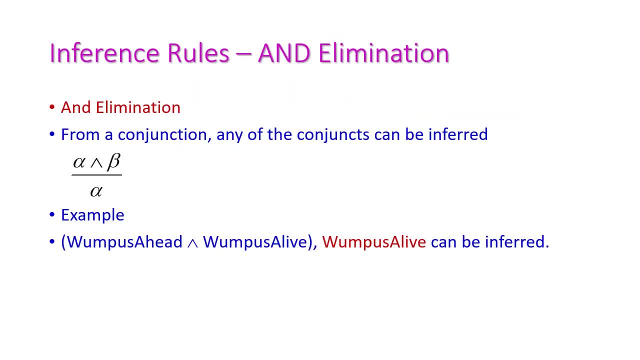 So the most important inference rules are modus ponens and and elimination. We are going to see these two things one by one. First, let us see the and elimination, That is, we need to remove this and operator from our The statement. Okay, 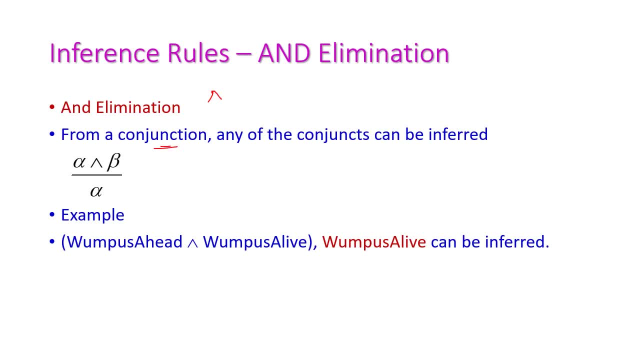 So the and operation is the conjunction. Any of the conjunct can be inferred. Okay, When we said this one is true. If alpha equal to true and beta equal to true, then we can say alpha and beta is equal to true, Right? 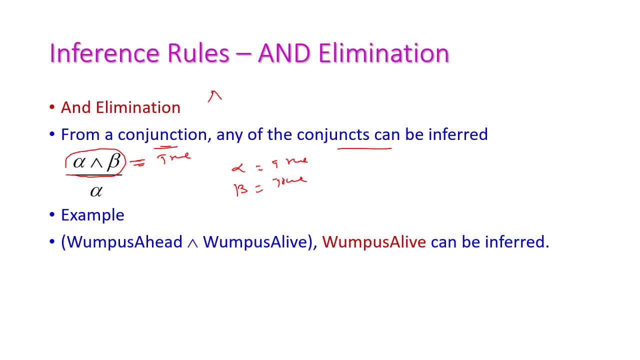 So, apart from writing this statement, because this is actually true, We have to write any one of This alpha or beta. Any one of these two will be taken. So the alpha and beta are the conjunct, For example, One plus ahead and one plus alive. 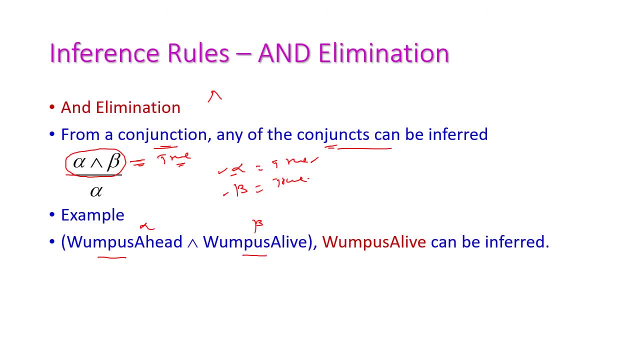 This is alpha and this is beta. So from these two statements we are going to take only this one plus alive, because both the things are true. Then one plus alive, Definitely True. So instead of writing everything, we can take only this particular thing. 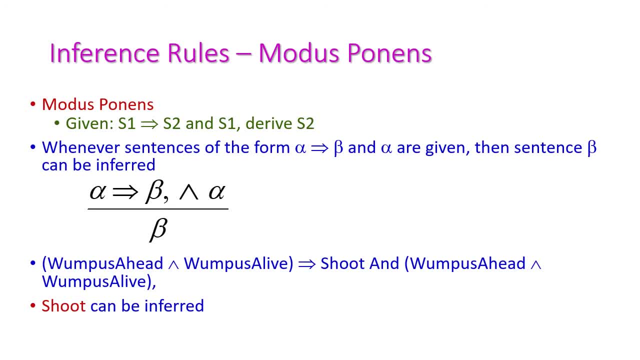 This is and elimination, And the next one is modus ponens. Next important inference rule is modus ponens. So here Given S1 implies S2 and S1. That derives S2.. Okay, Here for example we can take: S1 is alpha. 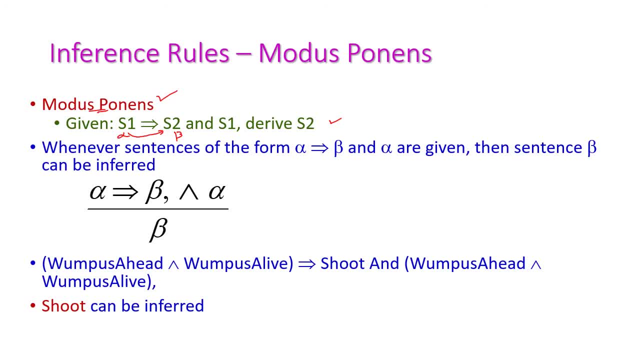 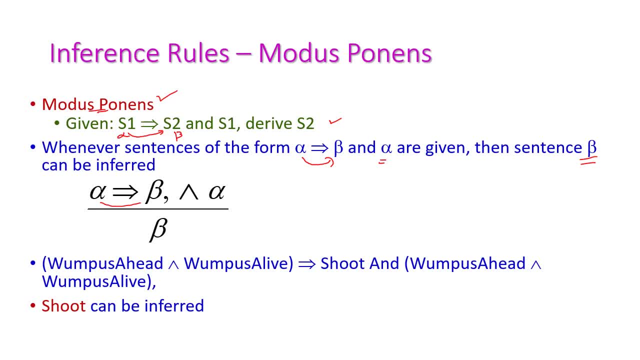 Okay, Alpha implies beta and alpha. Here we can infer only this beta, because whatever value the beta have, that only the output of this particular sentence. So we can directly take this beta Right here. one plus again: Right and wampus alive, which implies shoot and wampus ahead and wampus alive. okay, so here the entire. 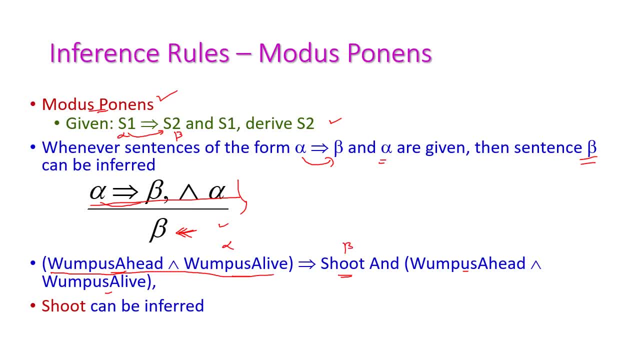 thing is alpha and the shoot is beta and the wampus alive and wampus ahead is alpha again. okay, so from this sentence we can directly take shoot. shoot can be inferred. instead of writing the entire thing, we can simply write shoot, right. so this is modus ponnel and this is the formula. 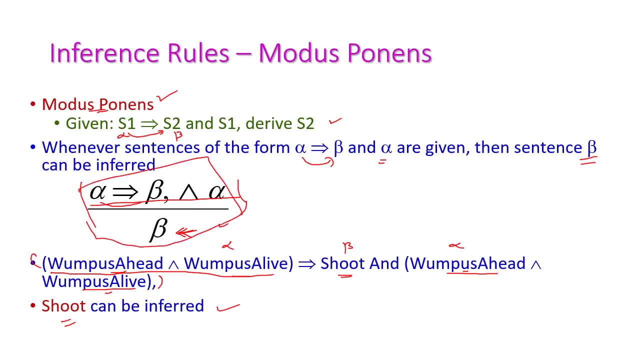 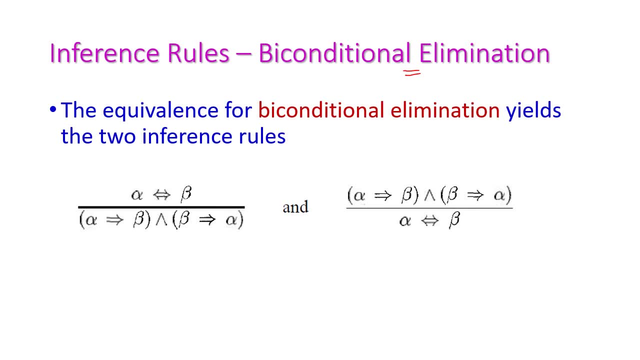 for modus ponnel. the another popular inference rule is biconditional elimination. okay, here the equivalence for biconditional elimination yields in two inference rules. two inference rules. first one is: we are eliminating this biconditional operator. how we are going to do this? alpha, biconditional beta. instead of this particular statement we can write alpha. 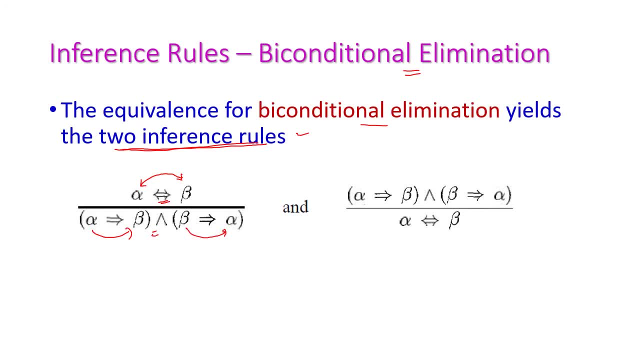 implies beta and beta implies alpha. right? so instead of writing alpha- biconditional beta, we can write this one. otherwise, in some other situation, instead of this particular statement, that is, alpha implies beta and beta implies alpha- we can write alpha biconditional beta. in both ways we can write right. so this is. 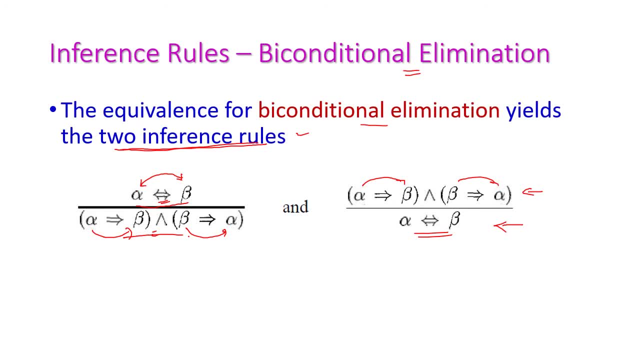 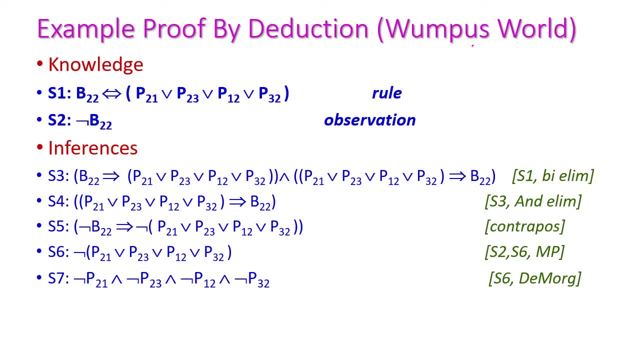 another biconditional elimination inference rule. now let us see one example for applying all our inference rules, and we can take our famous wampus world example again here. okay, in our knowledge base we are having two statements. okay, this is first statement and this is the second one, right? 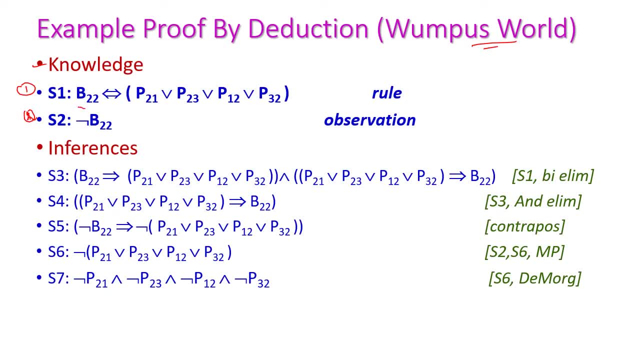 s1 is equal to bf 2 comma 2, biconditional pf 2 comma 1 or pf 2 comma 3 or pf 1 comma 2 or pf 3 comma 2. okay, and the second statement is not bf 2 comma 2, right? so here this is breeze. 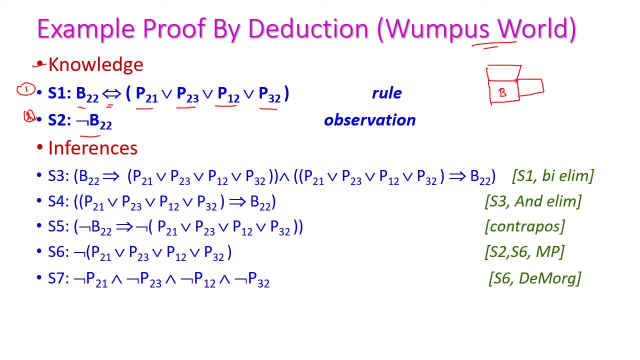 place and these are all the place of possible places of a pit. pit may be here here, here here, right? so this is 2 comma 2 and this is 2 comma 1. this is 2 comma 3 and here is 3 comma 2 and here is 1 comma 2. okay, 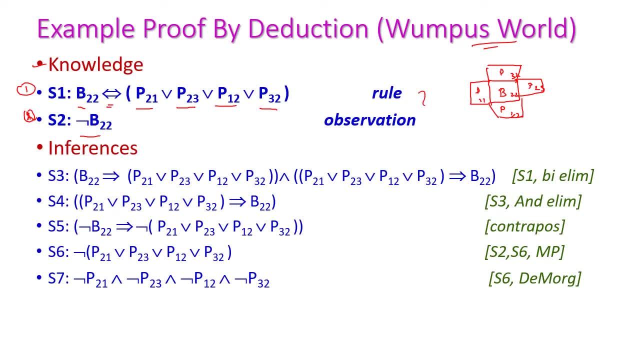 so with this rule observation we are going to inference the following thing: the first one is in the s1 statement. s1 biconditional operator is there, so we have to eliminate this biconditional operator from s1 so that we will get this s3. so how we are. 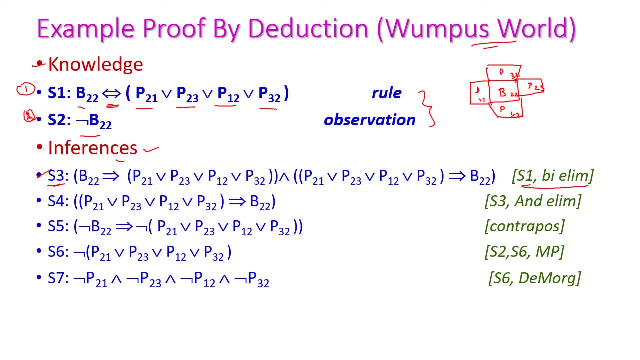 going to remove this biconditional operator by including. this implies operator and the and operator. okay, so for taking, this one is alpha and this one is beta. what is biconditional elimination? alpha implies beta and beta implies alpha. okay, b of 2 comma 2, which implies: 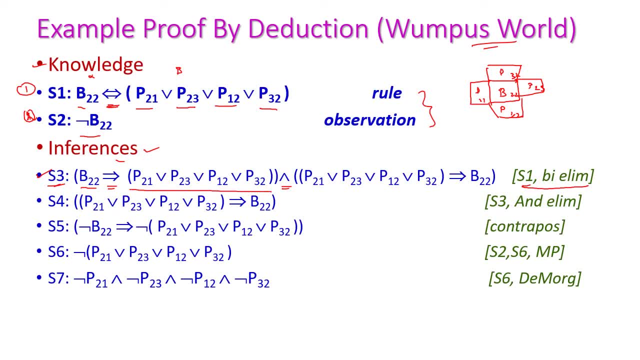 all these things, that is pf 2 comma 1 or pf 2 comma 3 or pf 1 comma 2 or pf 3 comma 2, and the same thing: pf 2 comma 1 or pf 2 comma 3 or pf 1 comma 2 or pf 3 comma 2, which implies bf 2 comma 2, so this: 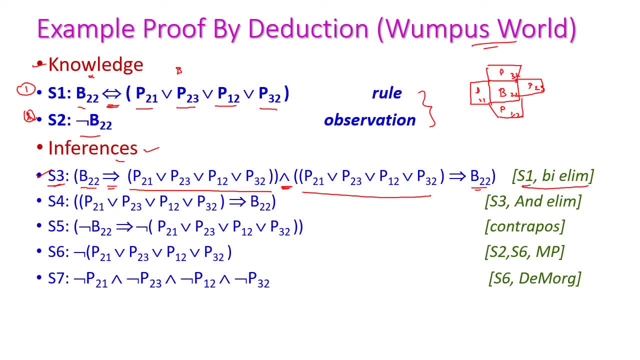 is biconditional elimination: s1 and from the next one and elimination will be there. okay, from s3. we need to remove this and elimination. right, We can take any one of this particular statement. So let us take this one and this will become S4, okay, So now S4 is PF2,1 or PF2,3 or PF1,2 or PF3,2. 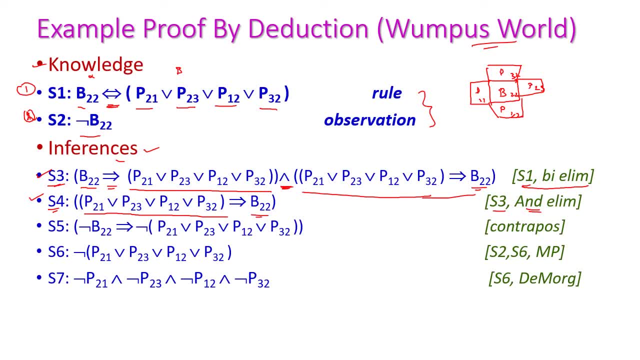 which implies BF2,2,. okay, Now we will get S4, right. And the next one is the contraposition. here The S5 is not BF2,2, which is implies not PF2,1 or PF2,3 or PF1,2 or PF1,3, okay. So this is contraposition. We are. 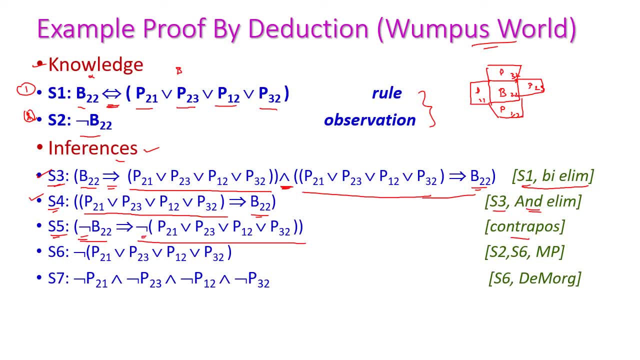 in P2,1.. So we have now S4,2,3,2,2,0,, BF1,2.. Okay, So this is irrequ존. So this is including this negation in both sides, right? so after that, the s2 and s6 will be what is this? 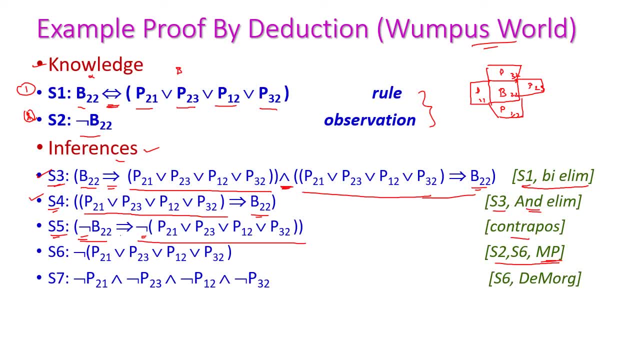 modus ponens. okay, here, this is implies operator will be there to remove this implies operator. we can apply this modus ponen. okay, so we can take this particular one right. this is s6. what is modus ponen? alpha implies beta and alpha, which implies beta, isn't. 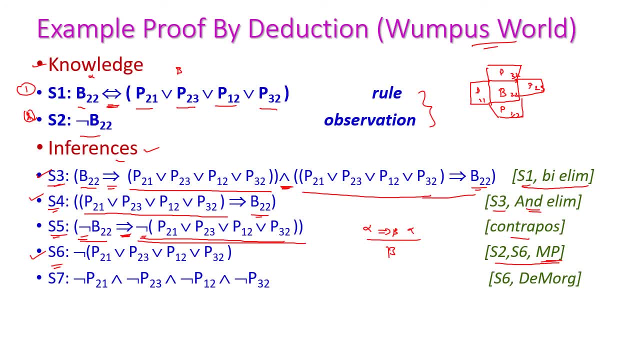 it so alpha again. alpha is here s2, so we can apply s2 and s6 with modus ponen. then we can infer only this: beta: what is beta here? not pf 1 comma 1 or pf 2 comma 3 or pf 1 comma 2 or 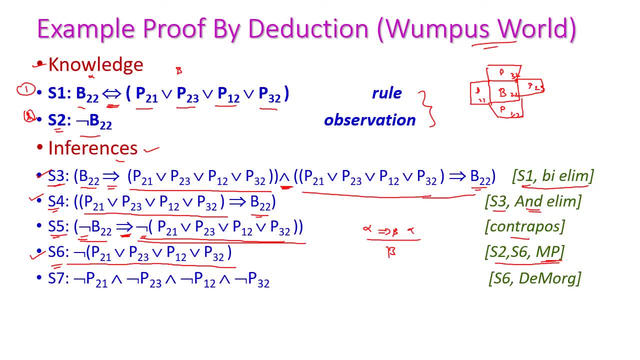 pf 3 comma 2. okay, then here we are going to apply the de morgan's law. okay, on this s6. then we can get this s7. what is s7 here? not pf 2 comma 1, not pf 2 comma 3, not pf 1 comma 2, not pf 2 comma 3. 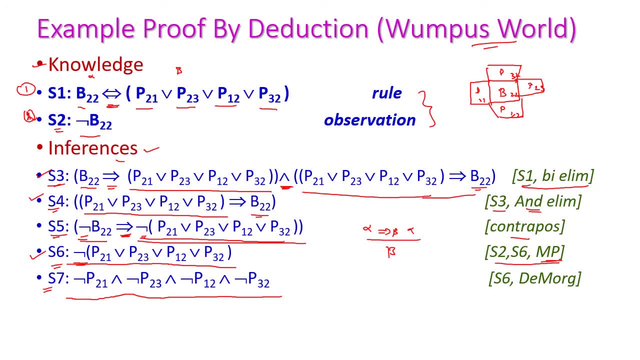 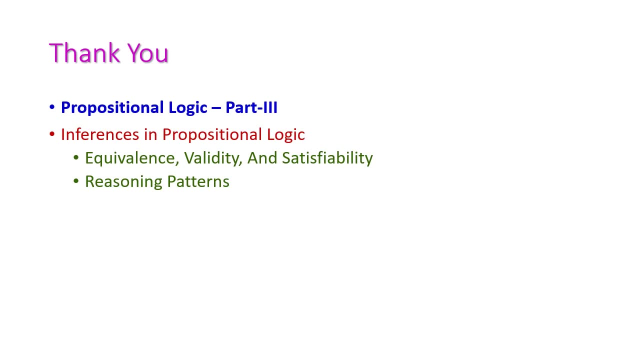 okay, so if it is not all these things, then there will not be any breeze in 2 comma 2. okay, so if it is not all these things, then there will not be any breeze in 2 comma 1. okay, this is the area that we want to note.